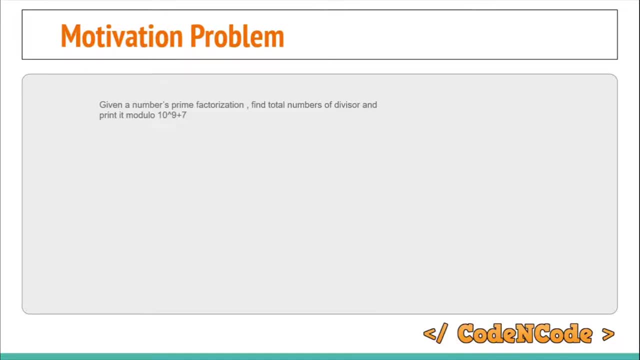 seven model is used is to counter the integer overflow, which means that the number, the result, is going to be too large, that integer overflow will happen. integer data type won't be able to handle it or won't be able to store it. so of course, the total 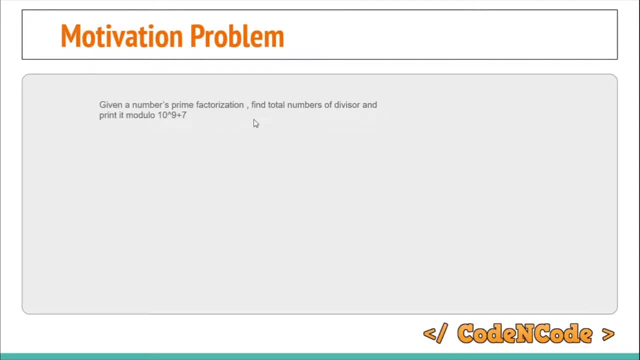 number of devices are going to be huge, so will you be able to apply square n approach and find all the devices? suppose this is the. this is the input of this problem. three means there are three primes and each pair is of the form p raised to power x. p is the prime number and this is raised. 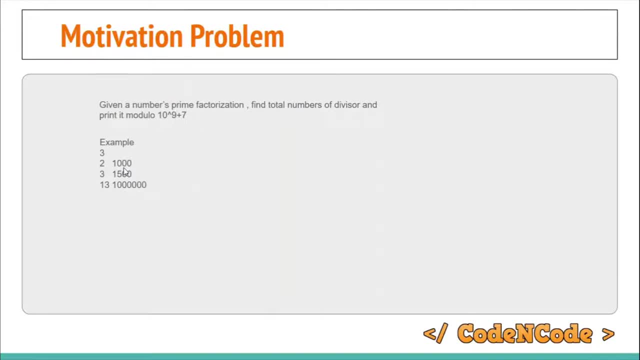 to power this. much so if, if i had to give input for number 12, i would give 2, 2, which means 2 raised to power 2 multiplied with 3, 1, which is 3 raised to power 1. so this is the number. the number is 2. 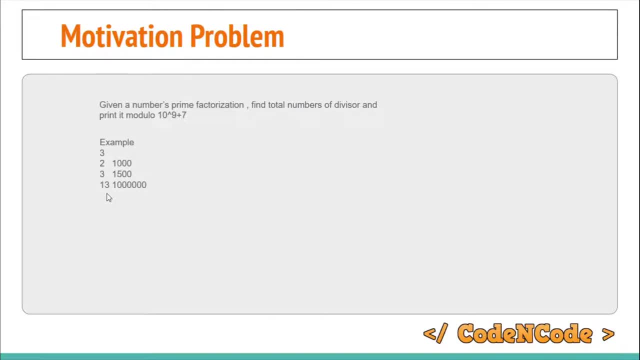 raised to power 1000 multiplied with 3. raised to power 1500. multiplied with 13 raised to power a million. so do you think you can create the number, the whole number, out of it and find the divisor in square root of n time? the answer is no, even if you are able to. 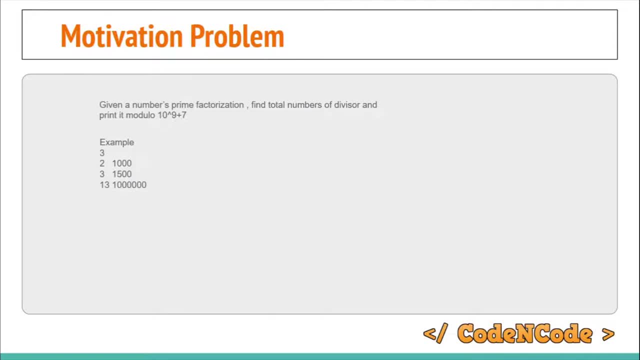 apply somehow square root n. you are 100 sure that, okay, square root of n won't result entirely, but is there any data structure that can hold this big number? remember, 2 raised to power 60 or 64 itself is so big that 2 raised to power 65 is so big that even the long, long. 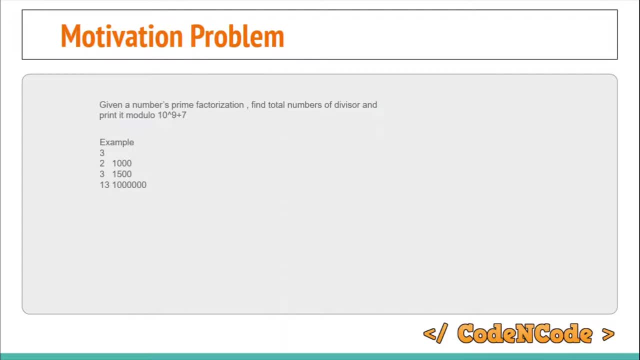 index will be able to hold this big number. so if you are able to apply somehow square root n data structure which is 64 bit, 64 bit data structure won't be able to store it. so how a data structure is going to store a number which is 2, raised to power 1000 only, but here 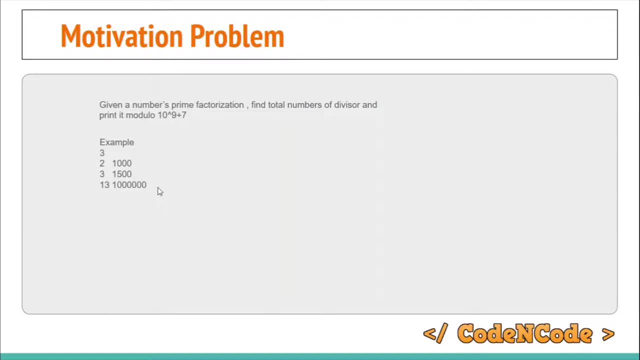 the overall number is much, much larger. so there is no way you can construct the whole number and then you can find the total number of devices of it. there must be other way around. there must be another algorithm, there must be other way to calculate the total number of devices of number. 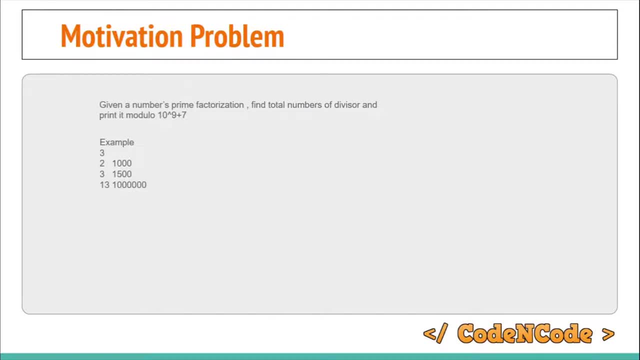 from its prime factorization, of course. well, the result is very easy. suppose we are given a number whose prime factorization is p p 1 raised to power y 1, p 2 raised to the power y 2, p 3 raised to the power y 3, dash, dash, dash. p n raised to power y n, when all the pi's here are prime numbers. 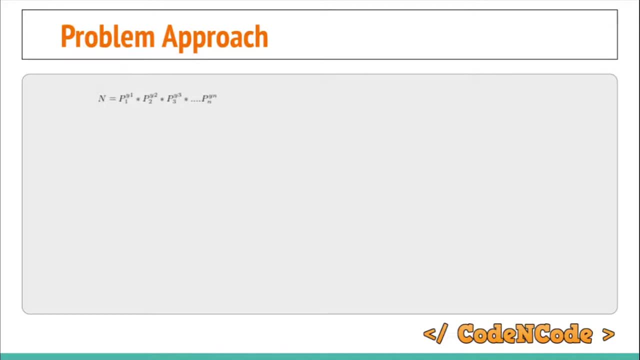 and y i's are their respective powers. so the total number of devices of such number is equals to y 1 raised. y 1 plus 1 multiplied with y 2 plus 1, multiplied with y 3 plus 1, dash, dash, dash, multiplied with y n plus 1. so if there are, 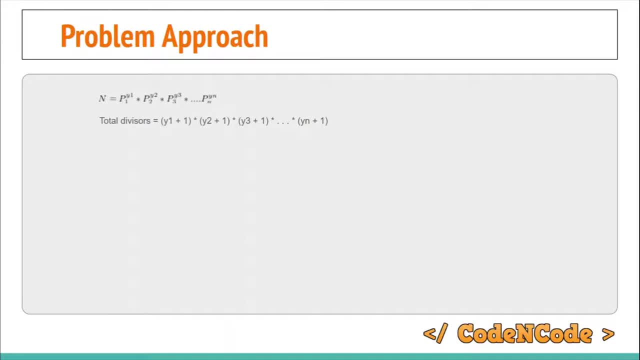 k number of times, then you can calculate the result: the number of devices in big o of k time. it is linear in k, the number of times, if take an example of 300. again, we knew that once the prime factorization with y, star, dash, dash will be played length into r by 2. 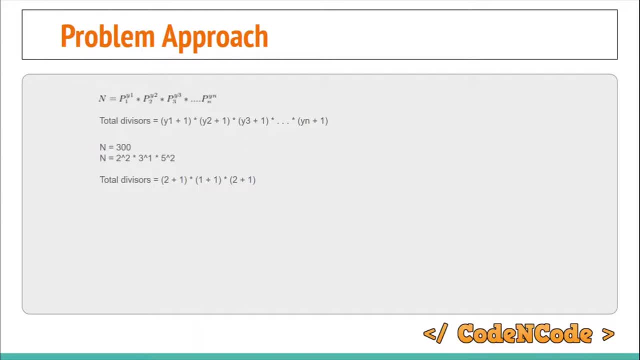 multiplied with 3, raised to the power of one, multiplied with 5, raised to the power of two, total number of devices would be two plus one, which is the first power, into one, plus i, which is again the second powerish, and again because it burdened or power. so the total number two. 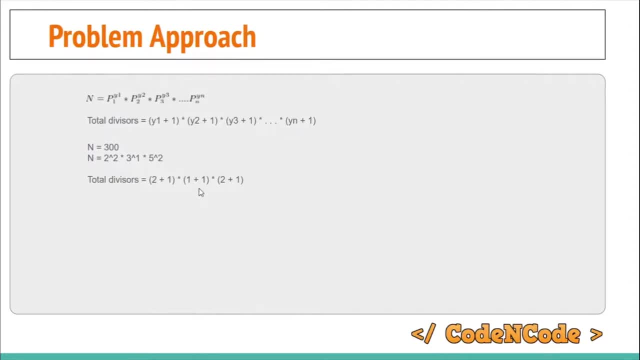 devices will be ninety to two. which is he head question is why this approach wants to be seen that. okay, the approach is very simple. all you have a have to do is take power of each prime prime factor and then add one it, one into it and multiply with. 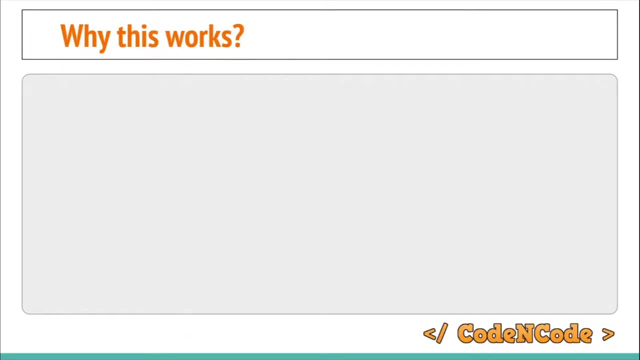 the already existing result. initialize result with one. of course, the question is why this would work. well, i will explain with a simple example, and you can extend or generalize this. let's take example of the same number again, and this time let's take three boxes. three boxes. 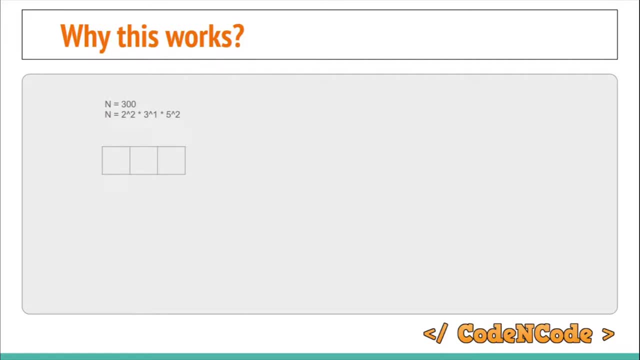 because we are having three prime divisors of n, one box for each prime number. first box is for two. second box is for three. third box is for five. now, what? well, now, what these boxes represent, you would understand with example. so in first box i have inserted one and then zero. in the second one, 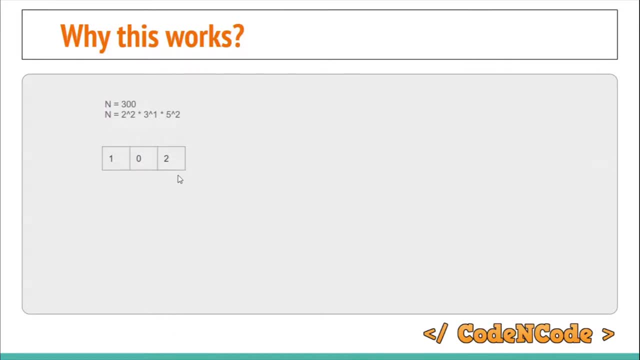 and two in the third one. this you can consider as a prime divisor because we are having three prime divisors of n, one box for each prime order and if you consider this box you can consider as a divisor generator. so what this number represent is actually this. number one means two raised to the power, one because the first box 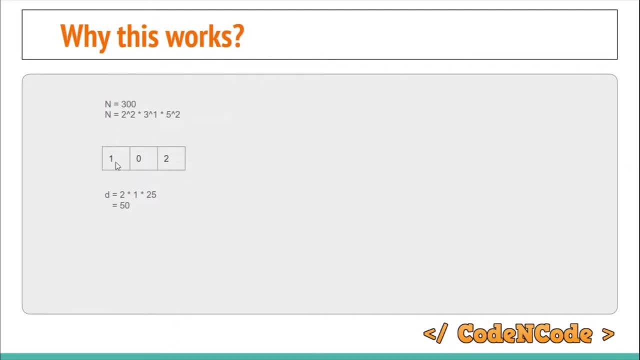 represent two. that is why one means two raised to the power one, and this actually represents their power. this three, this represents three, raise to power zero, and three is positive, is actually one and two, which means five raised to the power two. so two raise to the power one, which is two, three, 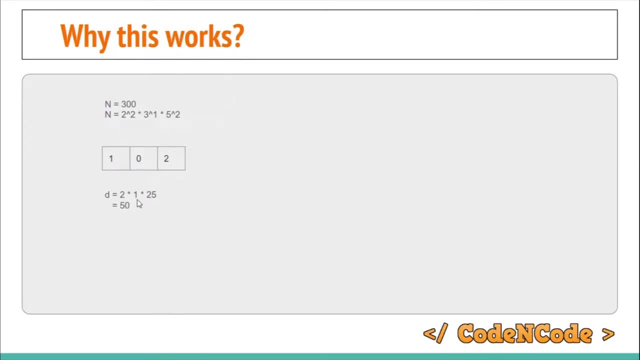 which is 1, 5 raised to the power 2, which is 25, so the overall result is 50. as you see, 50 actually divides 300, so this is a divisor. that is why i'm calling this box or divisor generator. now, uh, suppose instead of 2, i filled here 3, will the resultant number also divide? 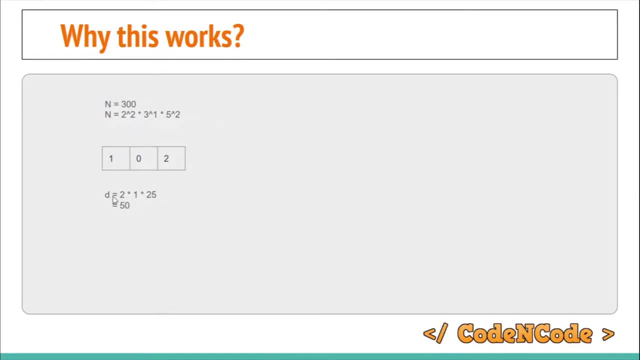 200, 300. the number would be: 2 raised to the power. 1 into 3 raised to the power. 0 into 5 raised to the power 3.. the resultant number won't be able to divide n reason this, which represent 5 raised. 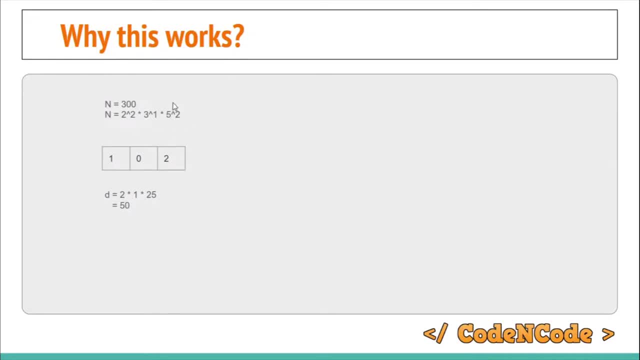 to the power 3 won't be able to divide. uh, this number won't be completely divisible by that, because in the original number n we are having maximum power of 5 as 2. so if a new number is having more than 2 of factor of 5 or more than 2 power of 5, then the original number n won't be divisible. 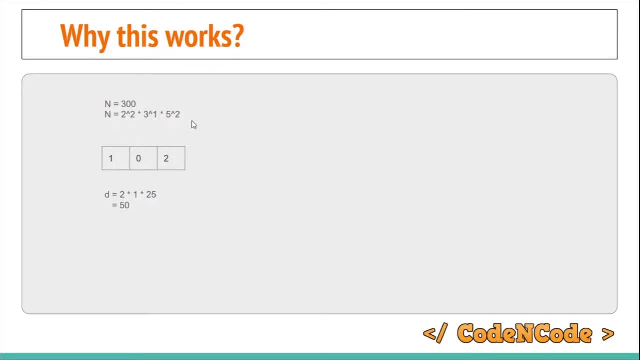 by that. suppose i'm dividing n with 5 raised to power 1, the whole number would be divisible by that, because 5 raised to power uh in in the prime factorization of n we are having 5 raised to power 2 and 5 raised to our 2 would be divisible by 5 raised to power 1, of course. so this would be. 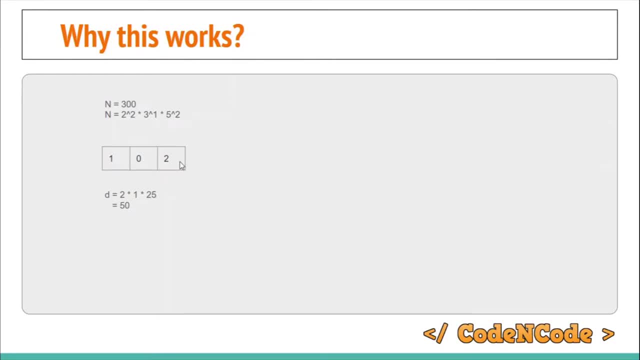 divisible. so if you fill at this place, at the place of 5, any number which is greater than 2, which means if you divide- uh, you try to derive a divisor in which power of 5 is more than 2, then the resultant number won't be able to divide n. this is not only for 5, but also for the every single prime. so if the 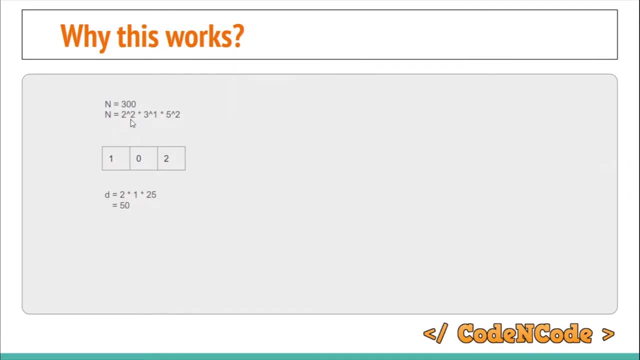 power of prime in the original number is x, then at the corresponding box you can't fill more than x. so you can fill, at this point up to 2, at this point up to 1, at this point up to 2. so first place can be filled in three ways. three ways because you can fill 0, 1, 2. second place can: 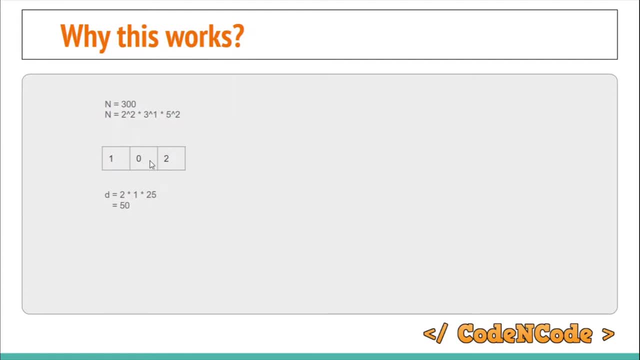 be filled in two ways, because 0 and 1. third place again can be filled in three ways: 0, 1 and 2. so the total number of permutation, or, sorry, total number of combination, would be 3 into 2 into 3, which is 18, and that is why all the total number of divisors are alpha of y, 1 plus. 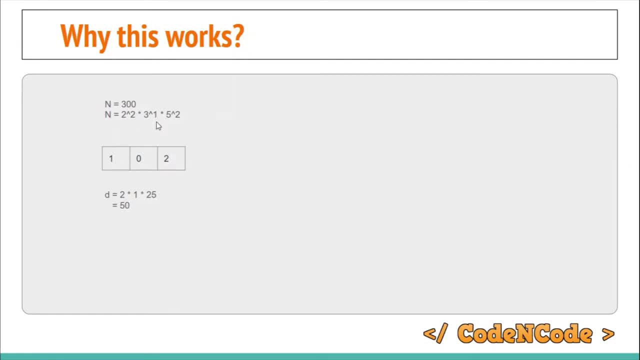 1, which is, of course, 3, into y 2 plus 1 and y 3 plus 1. that is why the formula works and the total number, the total number of combination, would be: uh, all would all will be unique. that is when a. That is why the total number of devices follow the formula that we have studied. 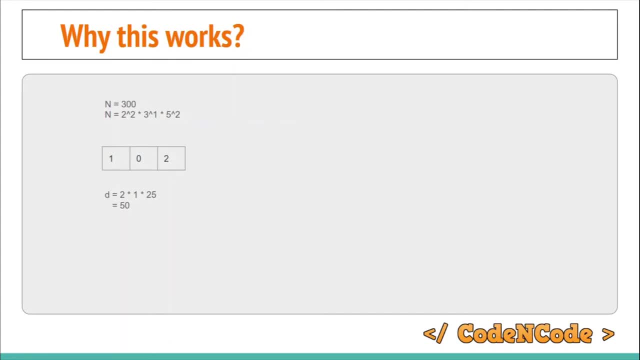 You can generalize this and you can google for the more concrete proof. This was just to make you see and believe why this formula actually works. Once you have something clear in mind, then even when you would go for studying the proof of it, you would be able to understand it more clearly. 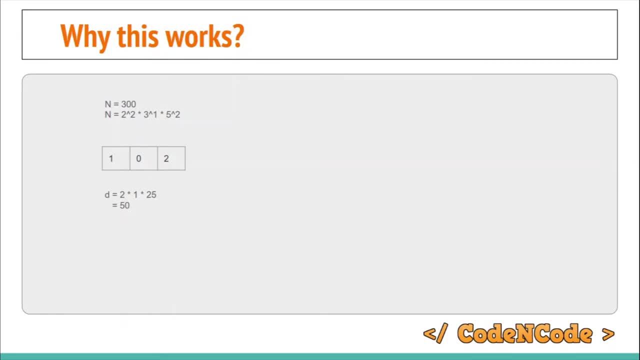 That is why I usually take examples to explain you, because it is important for you to at least have a clear idea why this works, and then you should go for the proof. So this was all for this lecture, and thank you guys for watching till the next video.